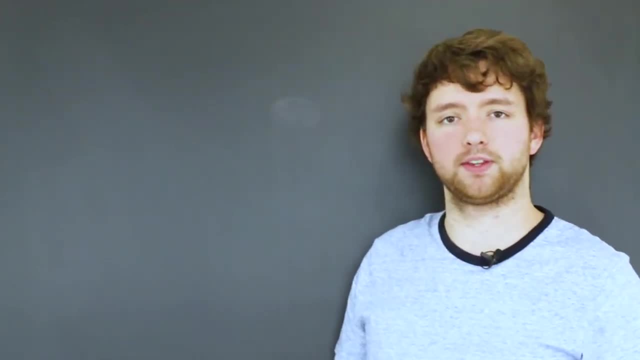 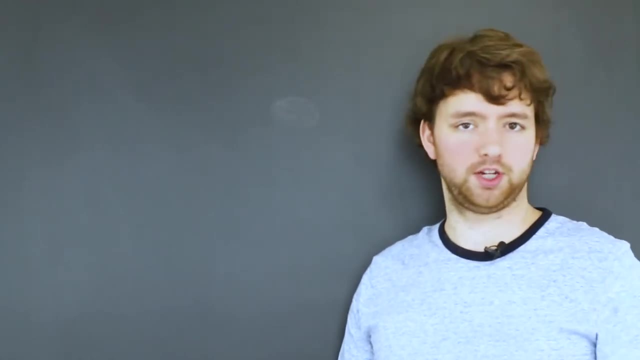 Yo yo, what's up? YouTube and other areas of the internet that find this video. Just wanted to say that this video is going to be about functions. Now, if you've watched this series from the beginning, you know functions. You got functions down good. 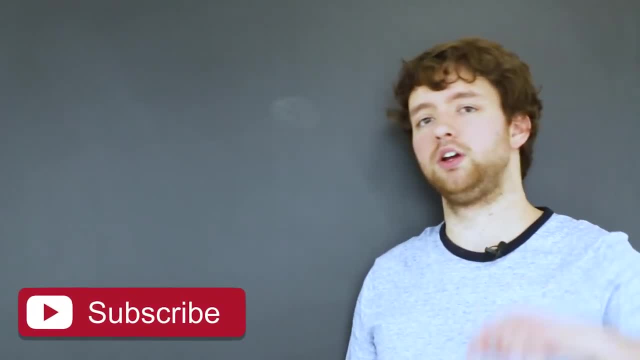 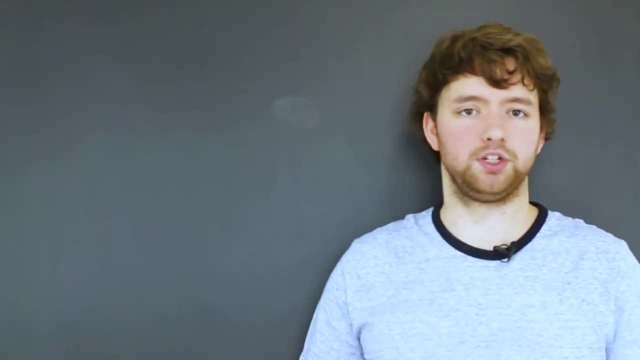 But I just wanted to go in more depth, sort of how I did a video on strings. even though we talked about strings, I wanted to talk about some of the principles behind functions and why you would want to use them. But just to review, let's talk about what a function is. 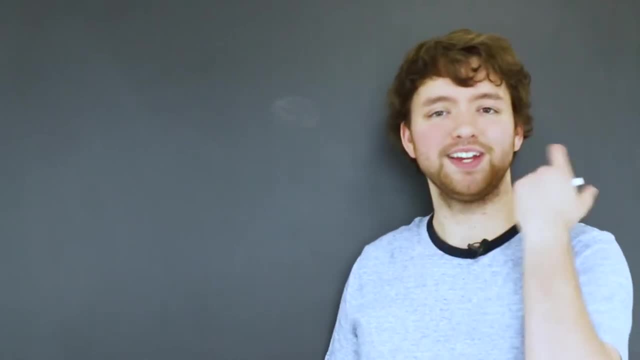 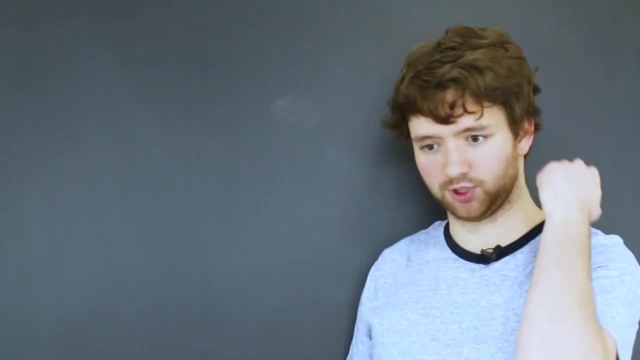 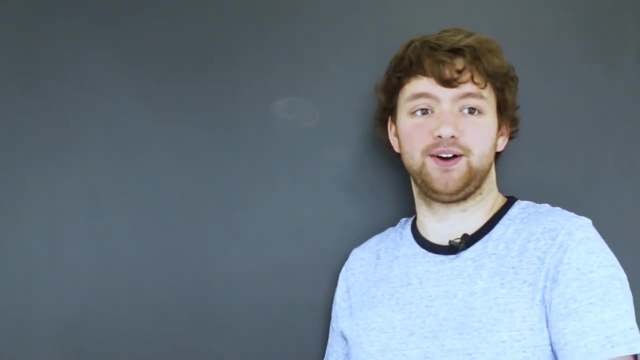 A function is basically you can think of it as a tool in your toolbox that does something for you. It's like- don't want to say slave because that sounds like really bad, But functions basically do the work for you and then you just call the function and you magically get an answer. 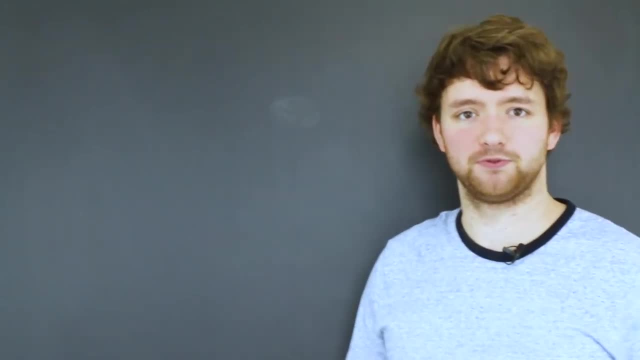 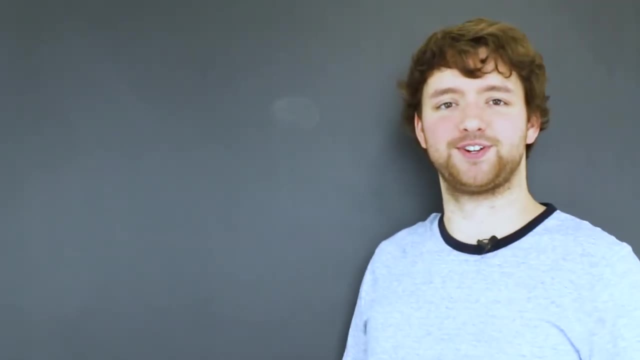 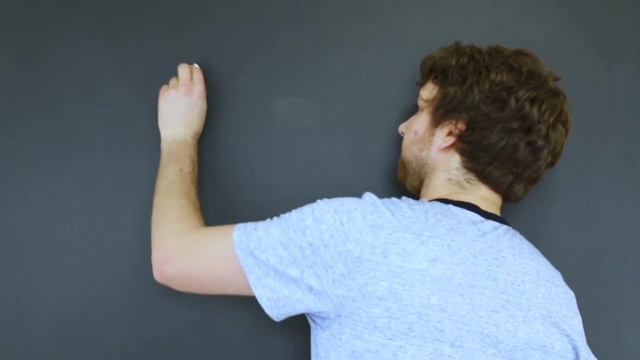 Slave was probably a pretty good use of The word. Okay, moving on into the less negative part of the video, What is a function? This is so weird. Okay, so a function. for example, we have printf, which is one of the simple functions we learned. 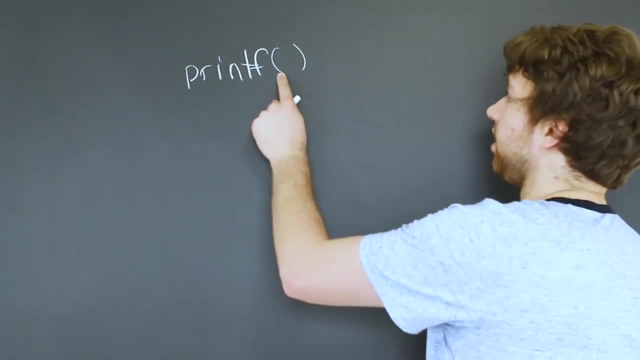 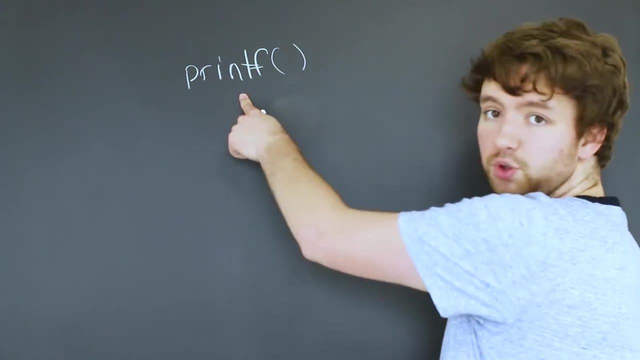 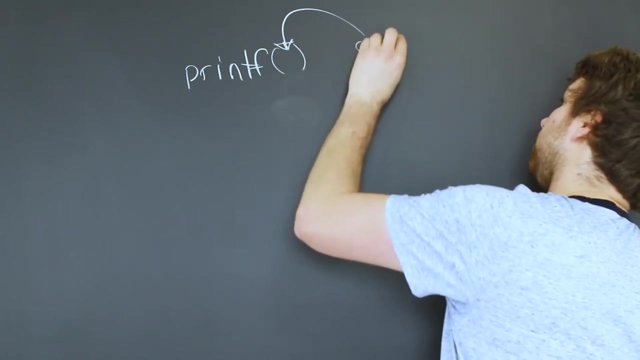 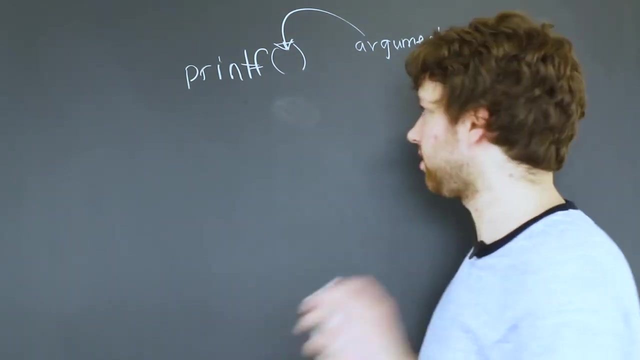 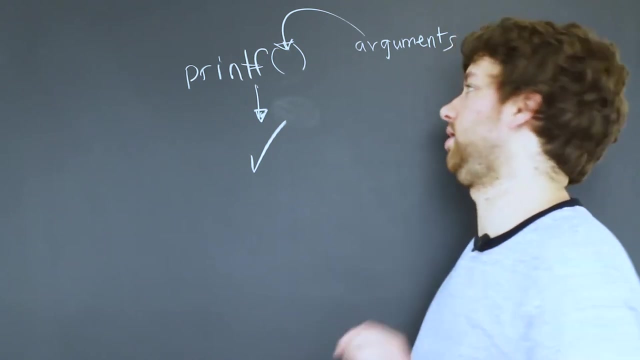 Functions have these. when you call them, you put these curly braces or the parentheses, And this all you have to worry About is what you put in here, which is known as the arguments, And you don't have to worry about how printf works or what it does, as long as the output from this function is what you want, which usually, if you are doing it right, it is because it's kind of like it's an agreed upon interface, in a way. 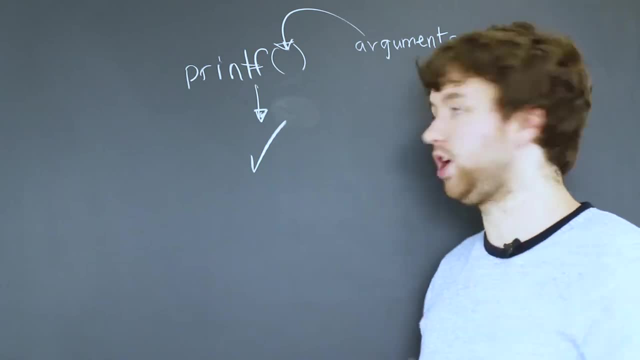 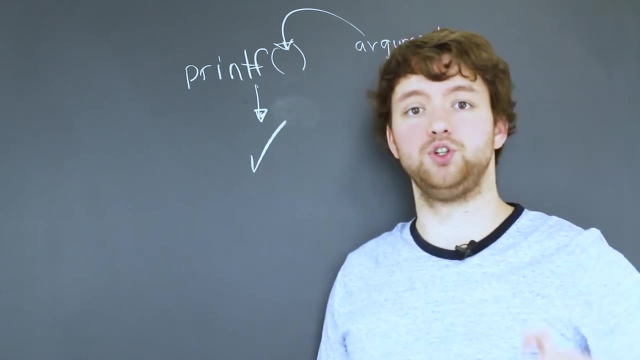 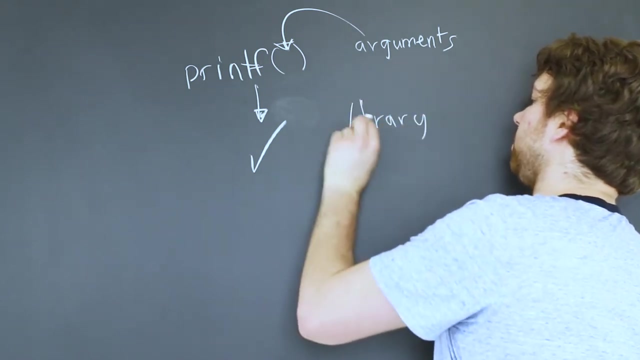 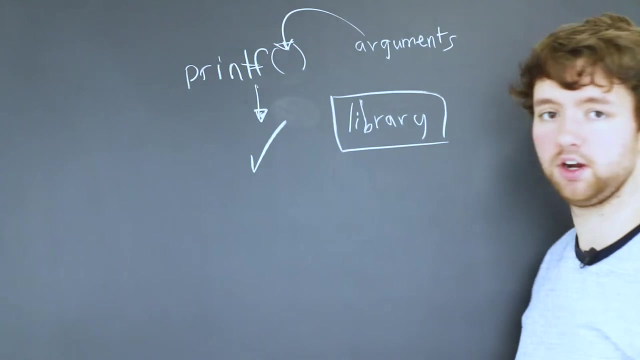 The arguments are the part you work About and in exchange you get an output That is the basis of a function, And you can create a bunch of these functions to do things for you and create a library. So we've talked about, you know, using the built in functions. but we can create our own functions and we can combine them into a collection known as a library. 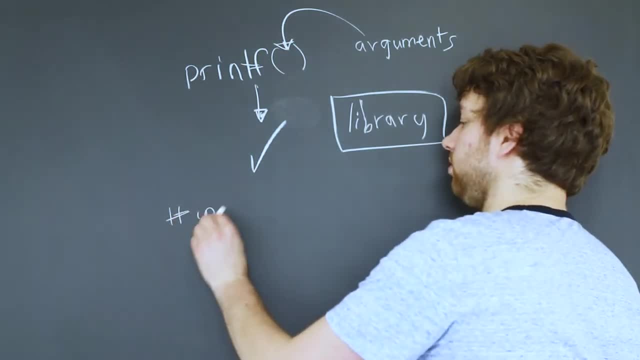 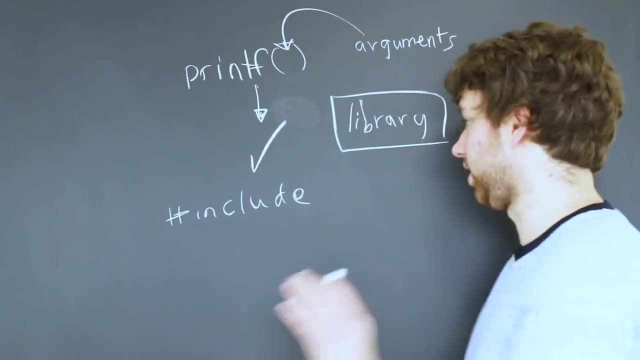 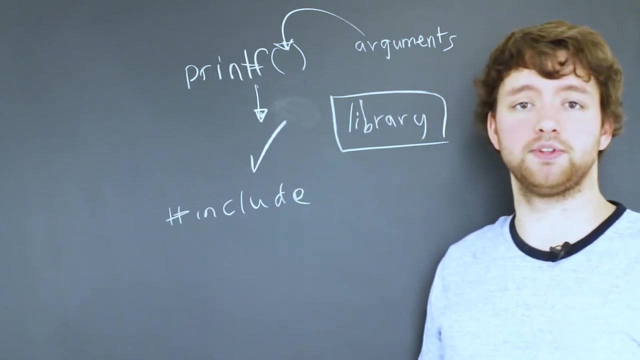 And then at the beginning of our program we can do an include sort of how we do like: include standard I, O, dot A, H or whatever it is standard bull. we can include our library and then have a collection of tools and our toolboxes, or you can think of it as weapons in our arsenal. 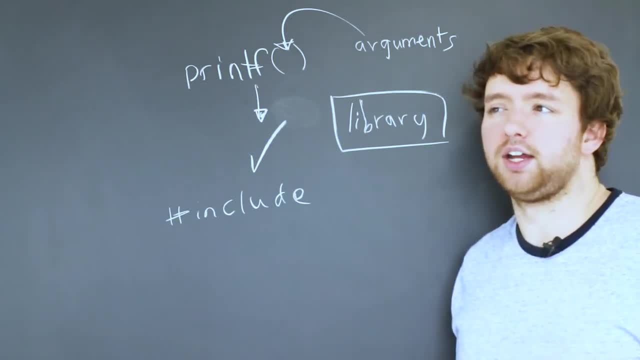 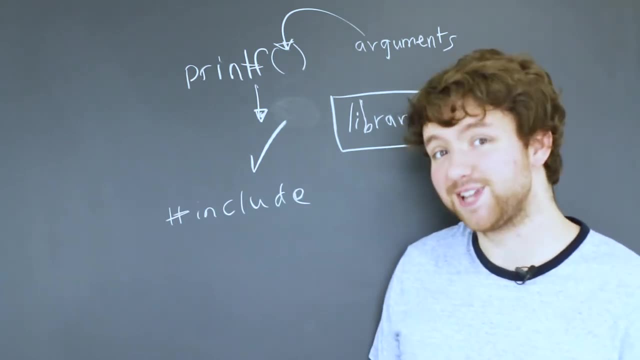 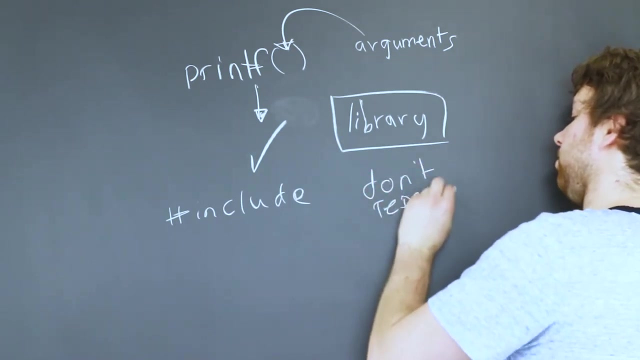 And, in general, you could say that the idea behind functions is very dry, because it stands for: don't repeat yourself, Okay. so yeah, don't repeat yourself. basically, if you have a piece of code that you're going To, 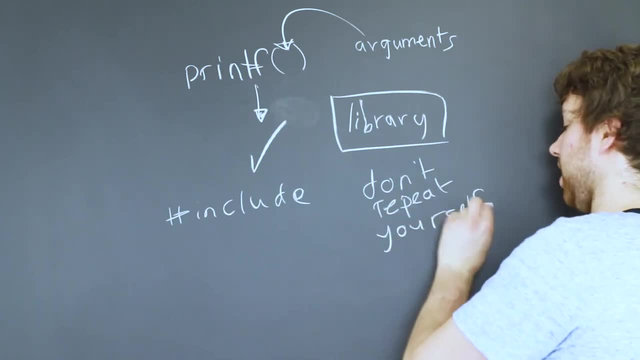 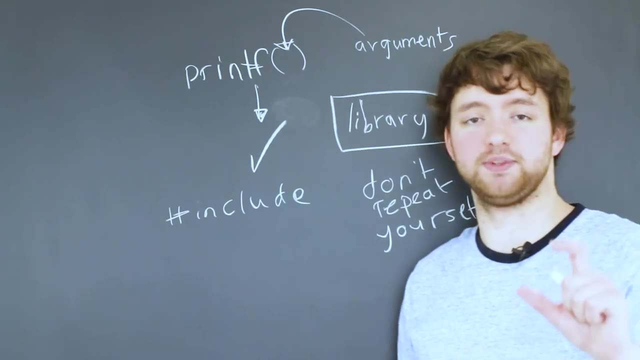 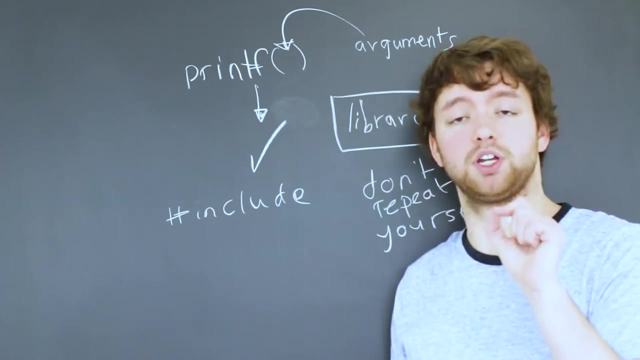 Call or do multiple times, you will definitely want to use a function because that reduces errors. It reduces mistakes, logical errors, So because if you were like, oh, this function is not working or the section is not working, quite right, you can go modify it. 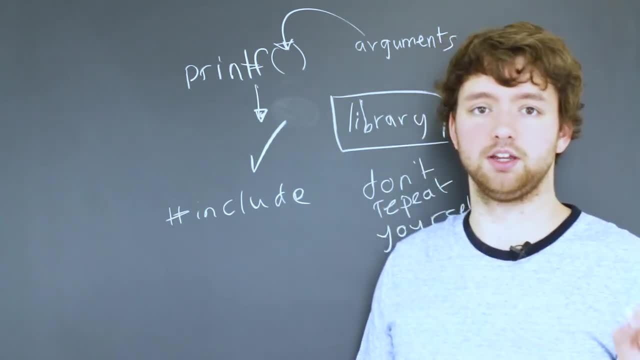 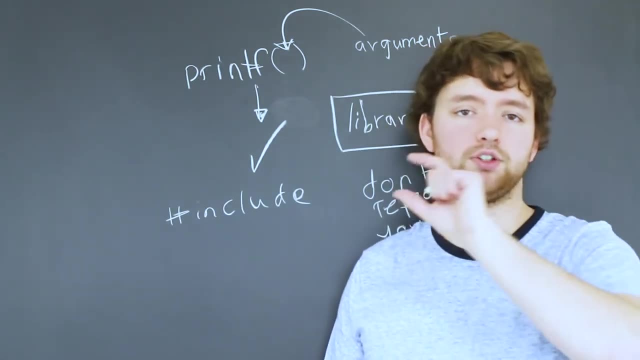 But you'll have to go remember to modify it in every location that uses it. But if you have a function, all you have to do is change the function code And, as a result, It's going to use that code every time you call that function. you can kind of think of it like Legos, right? 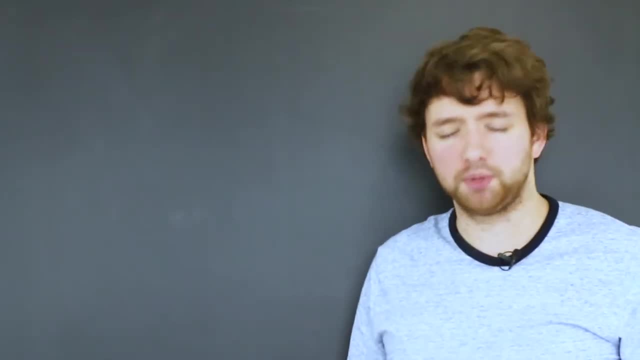 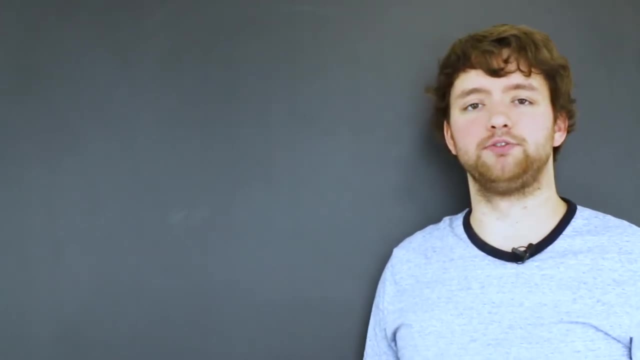 So these functions are Legos. right now We're just working with like pure plastic and we are building applications using custom plastic. but it would be so much easier if we formed Legos out of this plastic And then we just had building blocks to make our applications. 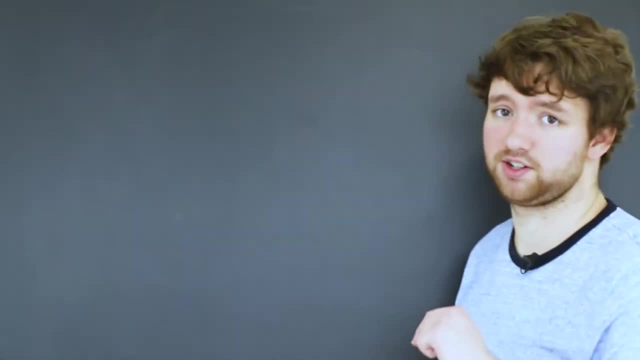 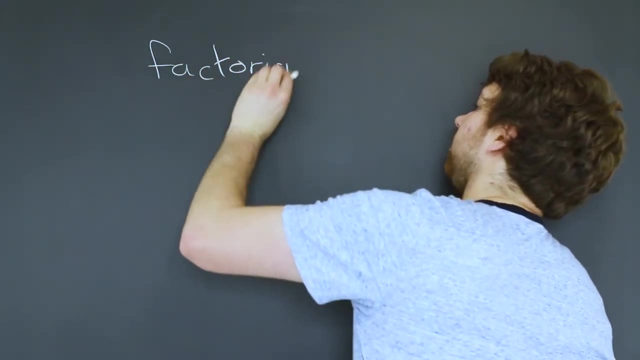 It's a terrible example. It's a terrible illustration, but it works. So, for example, we could create a function factorial, And maybe something like this already exists and basically, in math, the factorial is when you take a number and multiply it by all the numbers lower than it. 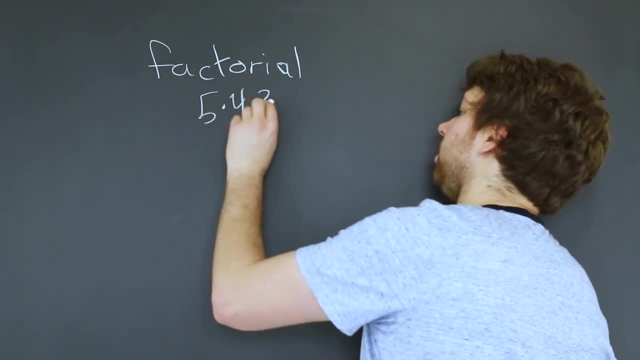 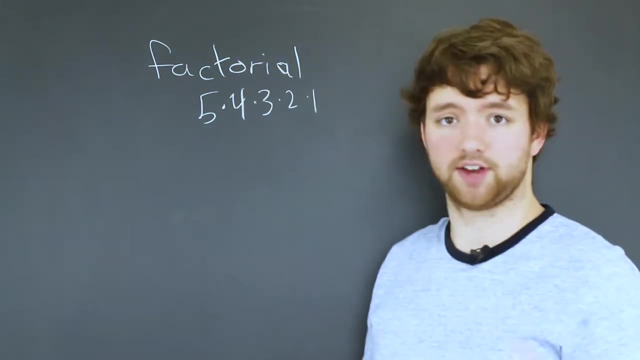 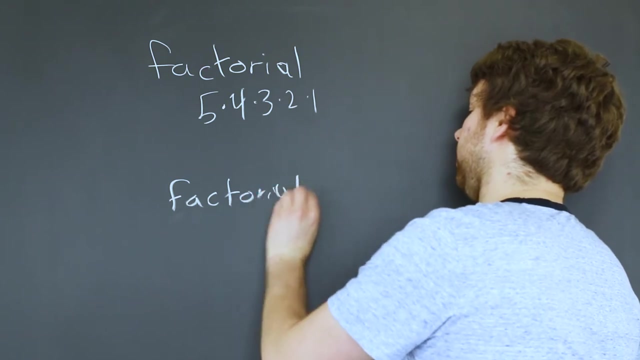 So the factorial five is equal to five times four times three times two times one, and we could manually calculate the factorial every time we need it, or we could just say factorial and pass in a five, and then this would return an integer. So 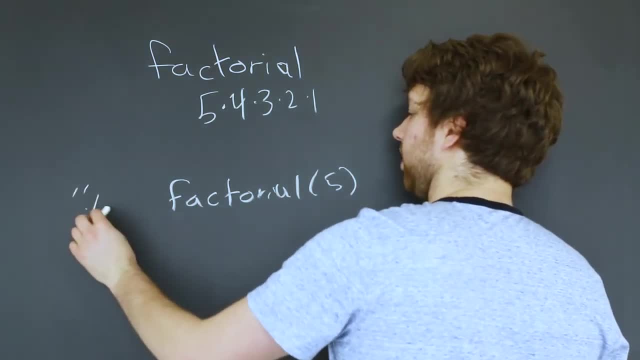 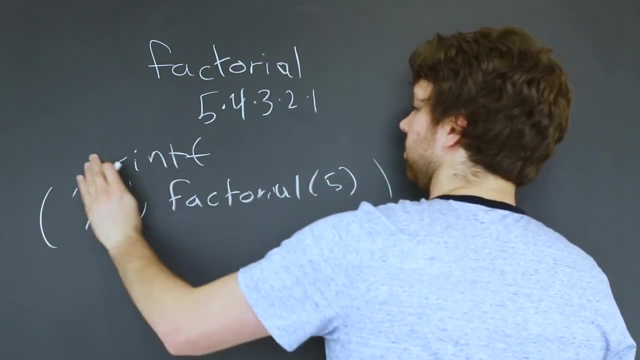 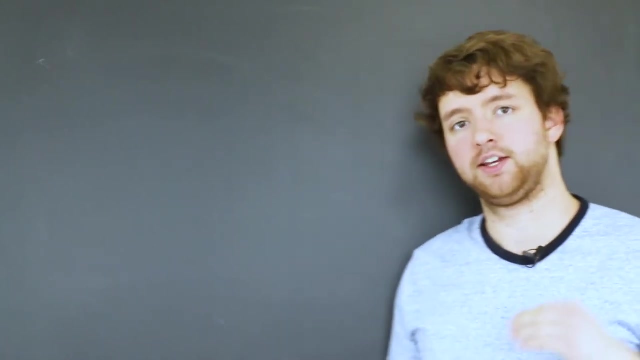 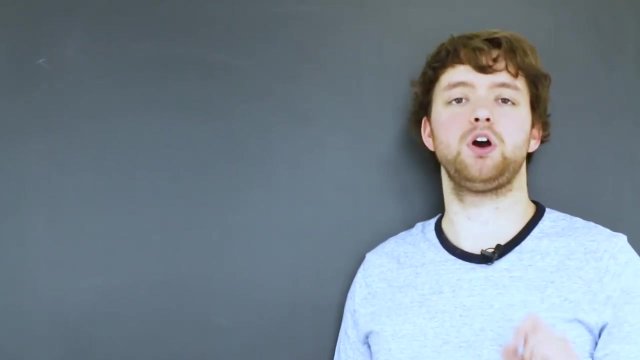 We could literally use this as an integer, So, for example, we could print it inside of a print F like such. Now there are some general things you should understand about function design, and there's just some good rules, right. So the first thing is that you shouldn't output to the console inside of a function. 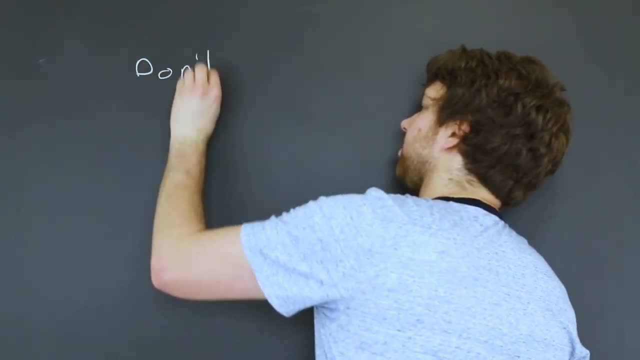 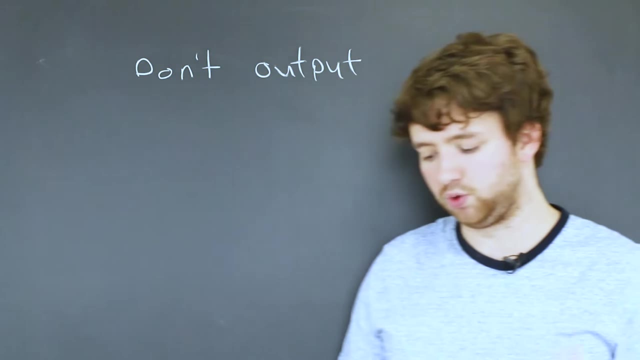 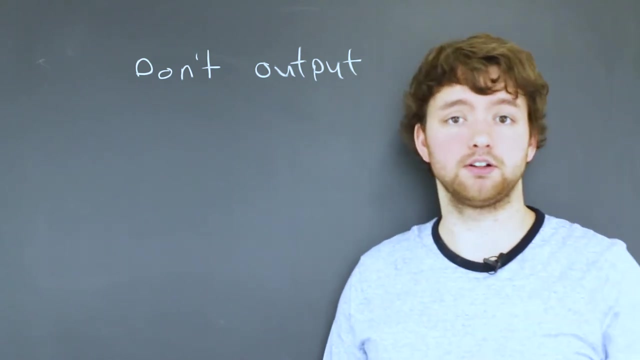 So don't output. And There's one exception, and that exception is if you wanted to do some kind of function that would do an elaborate print, a set of prints, to basically log a series of data in the console. So if you wanted to make the printing process easier, you could create a function to do that. 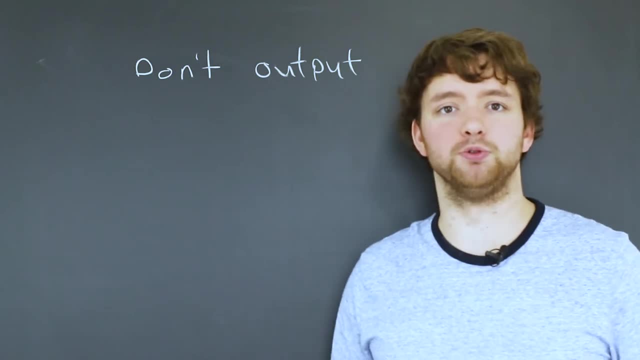 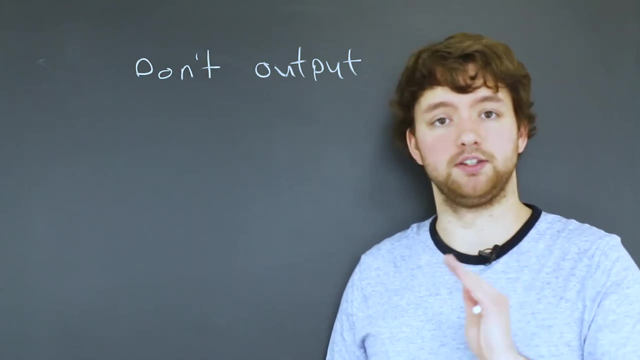 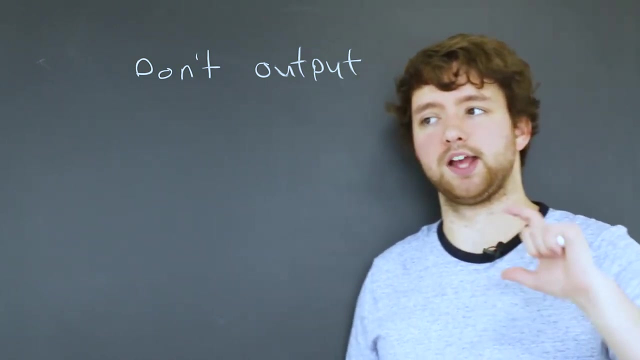 You could just call it like output or dump variable values, or whatever you wanted it to do. Um, but in In functions that aren't specifically designed to output data, you don't want them to output data because it limits the use. You want the function to be as general as possible so you can use it in more than one scenario or scenario. 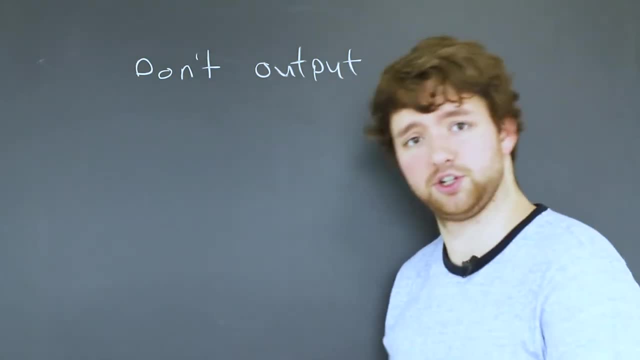 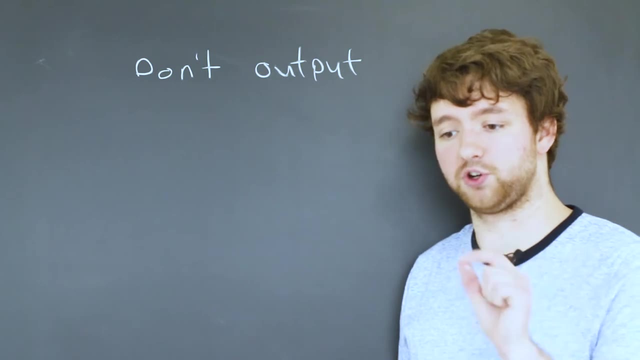 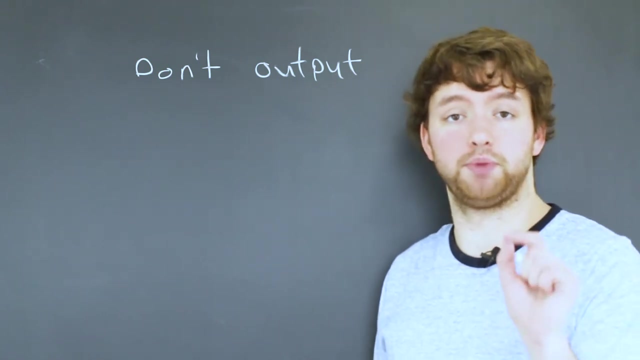 Do you guys say scenario or scenario, Just curious? So don't output. That means, if you, um, if you want to create a function, Uh, the output, The output, The output would be in the calling side. So let's say we wanted to compare two variables. 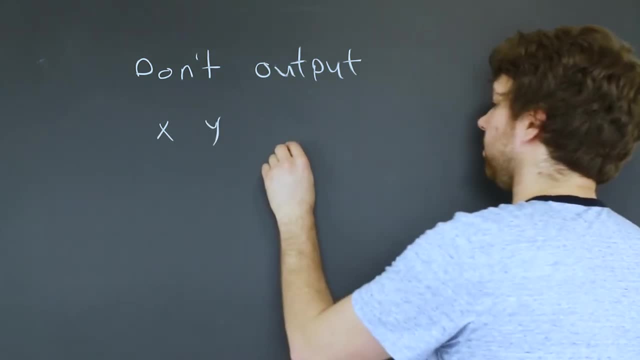 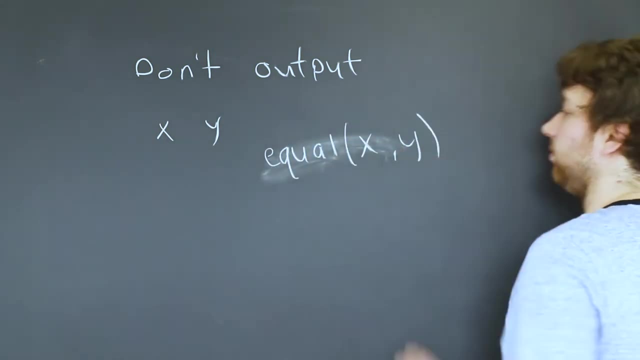 Let's just say we have X and Y and we have a function like I don't know, are equal. We'll just call it equal And you pass in X and Y and then you could throw this function call inside of an if statement. 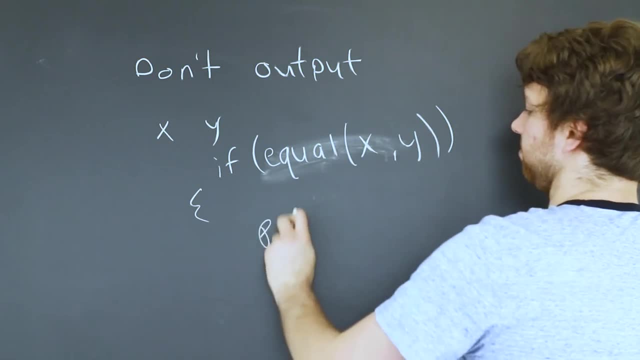 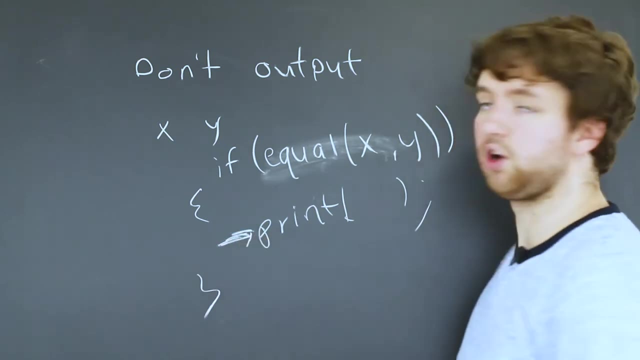 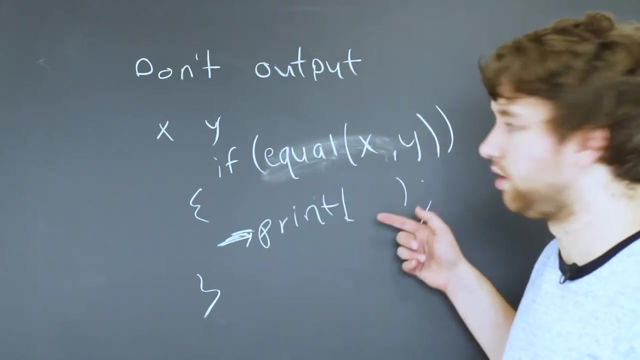 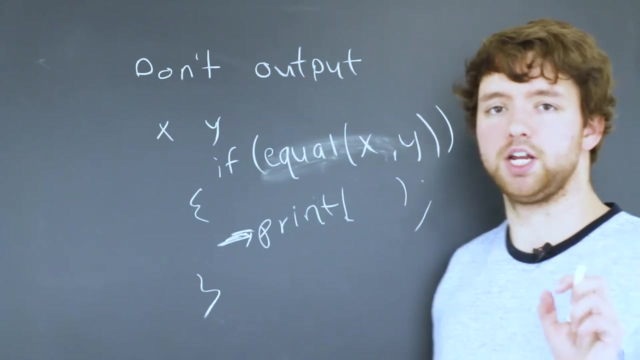 So if equal, And then you could print something Whatever you want, You can do the print In the calling side. So the calling side is we're, we're calling this function and we're printing based on the results. Some people instead would inside of the equal function that they defined. if they're equal, they would print inside that function and say they're equal. 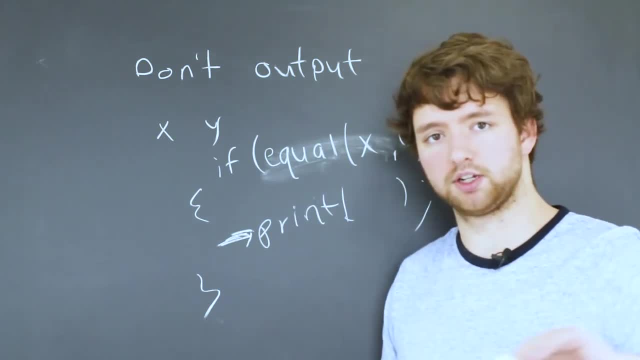 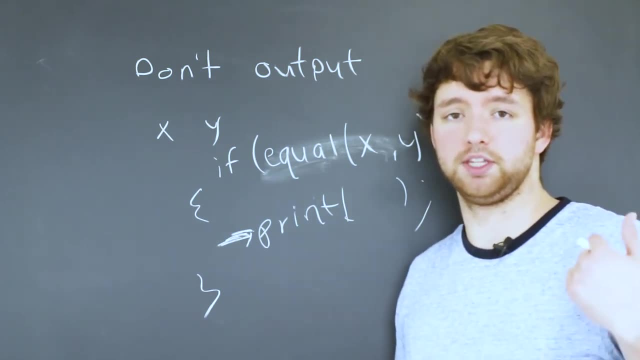 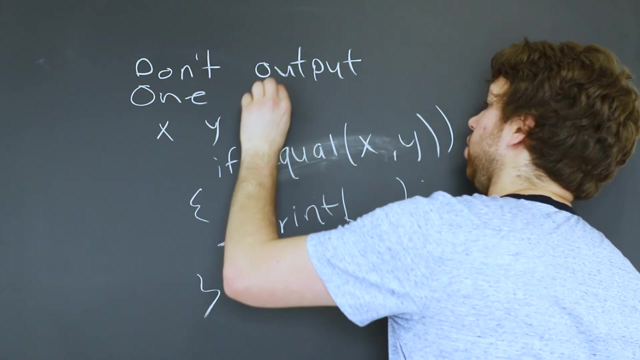 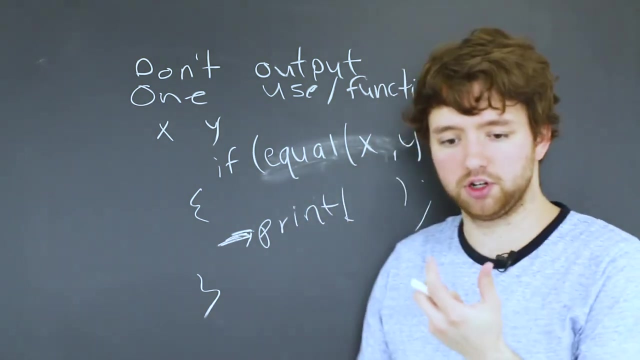 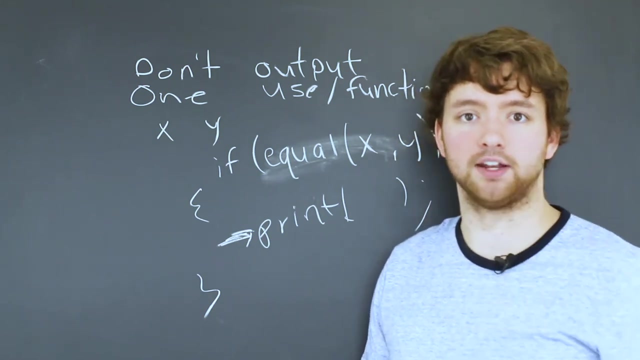 But that means every time you use this function, even if you don't want it to print, it's still going to print. They are equal. So you want to basically extract anything that's going to limit the use of the function. Another good rule is um you try to make the functions have one use or one function, basically meaning that the function, um the name of the function, should describe what it does, and it should not have the word and it should do one thing. 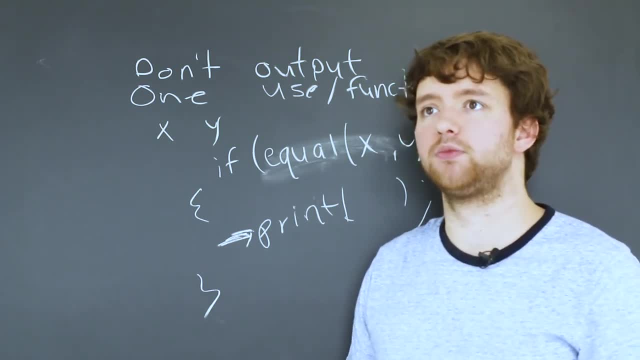 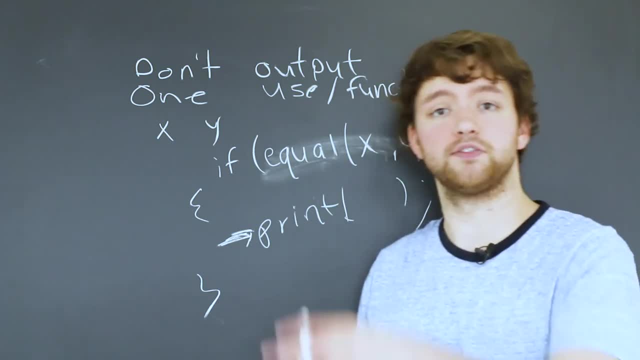 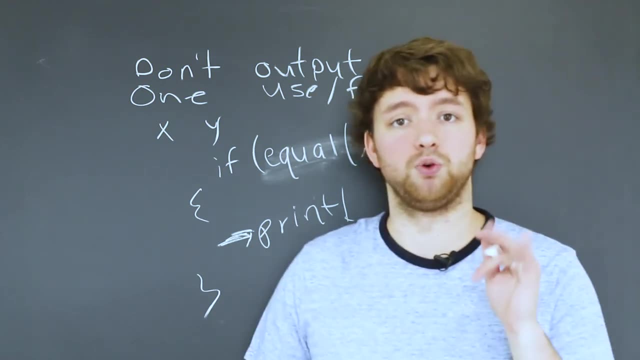 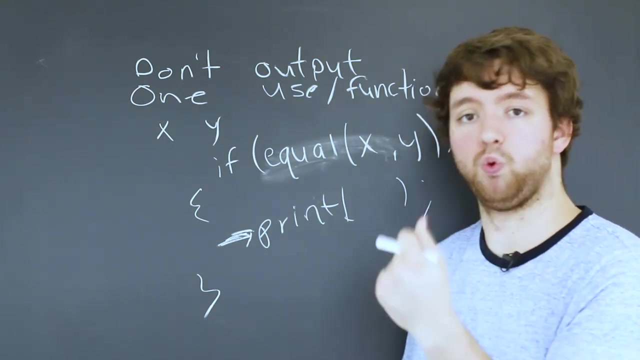 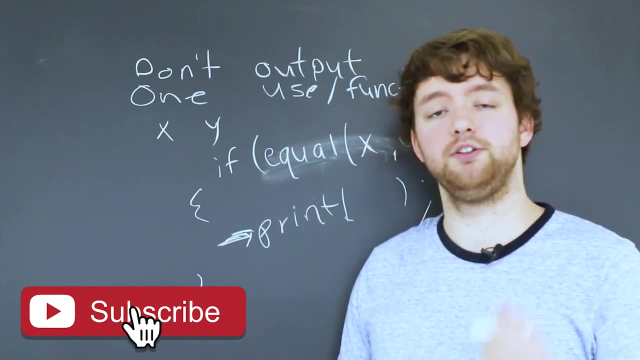 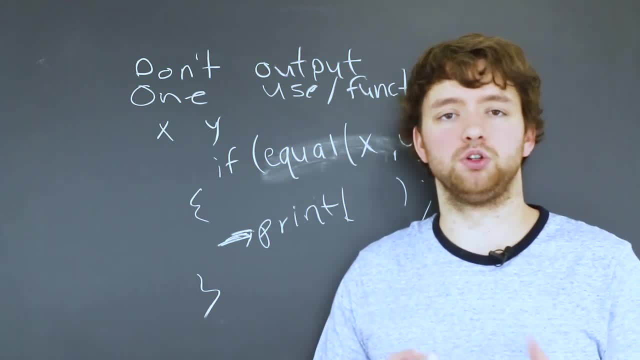 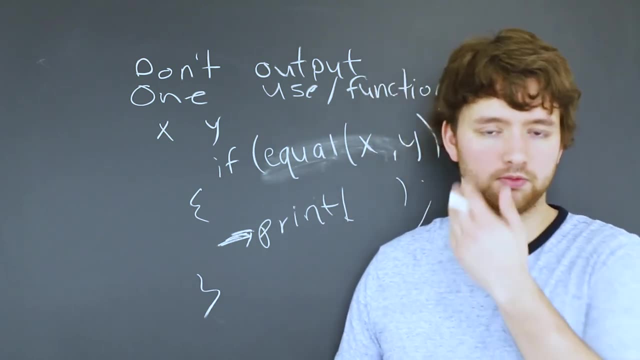 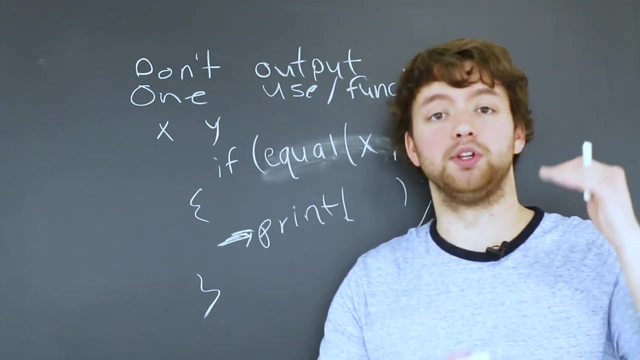 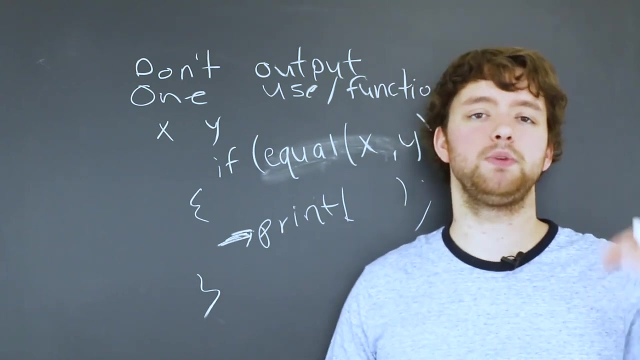 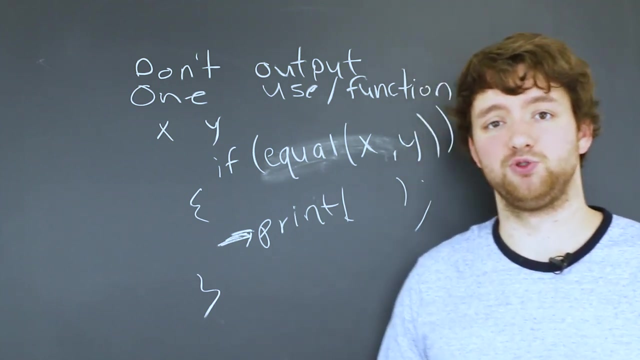 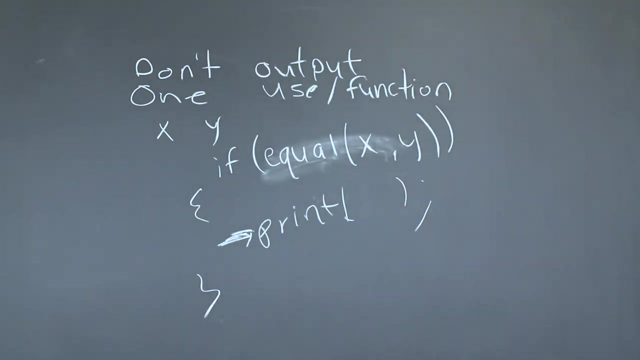 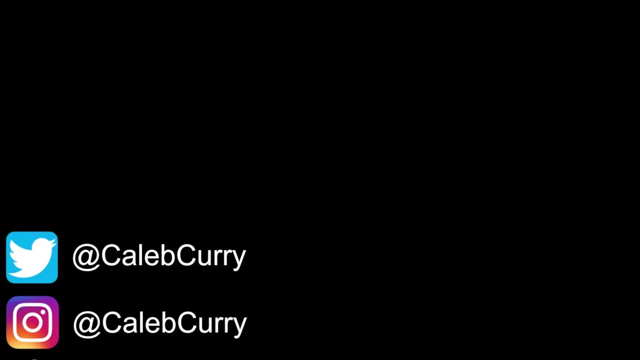 Okay, Okay, Okay, Okay, Okay, Okay, Okay video. please be sure to subscribe and also check out the the crash course in the description below. see ya, you.